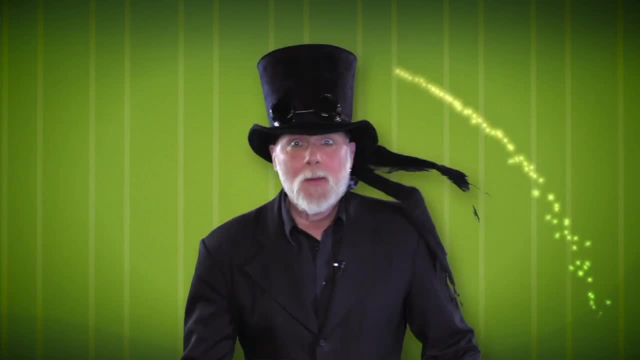 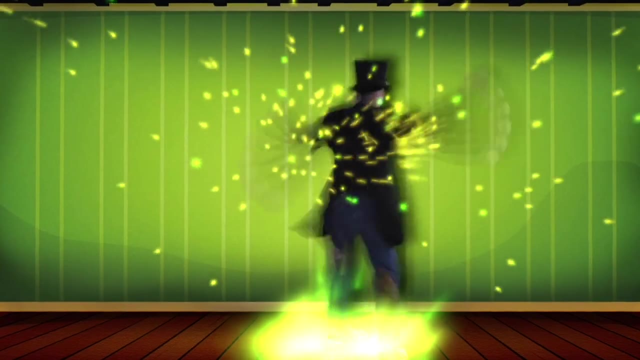 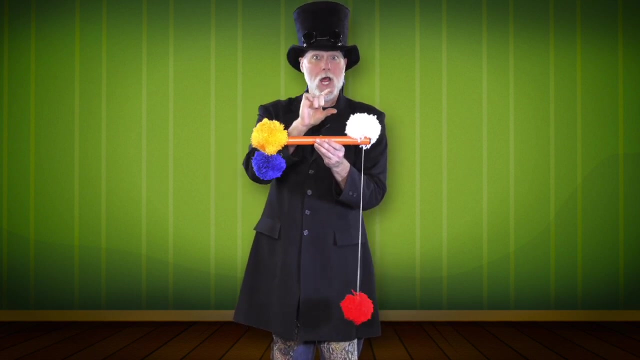 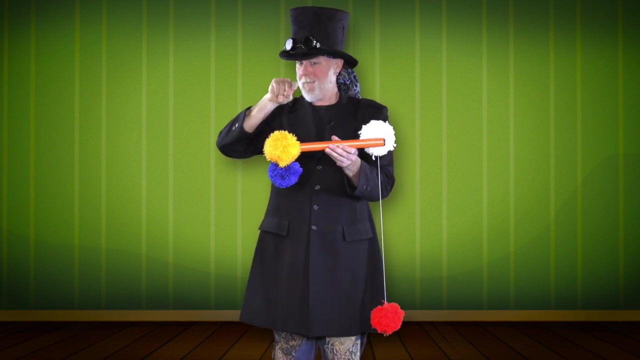 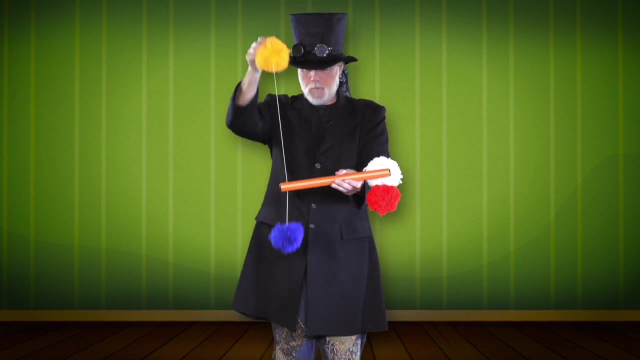 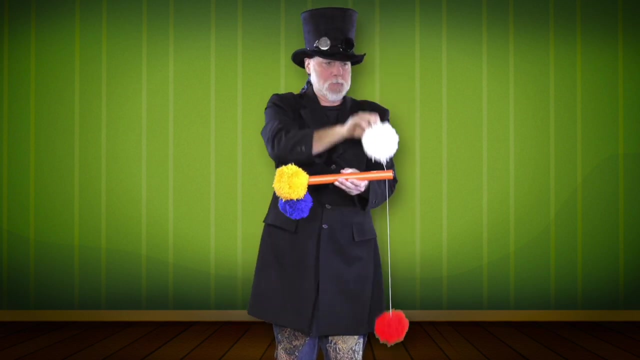 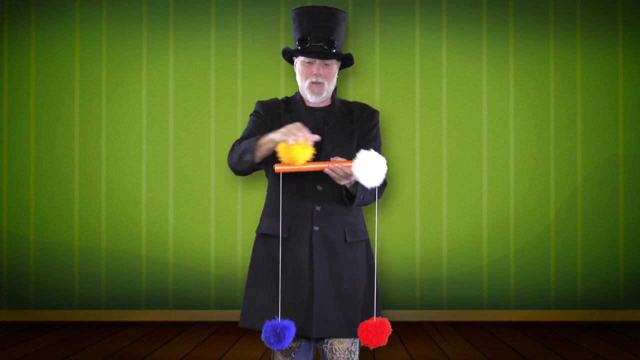 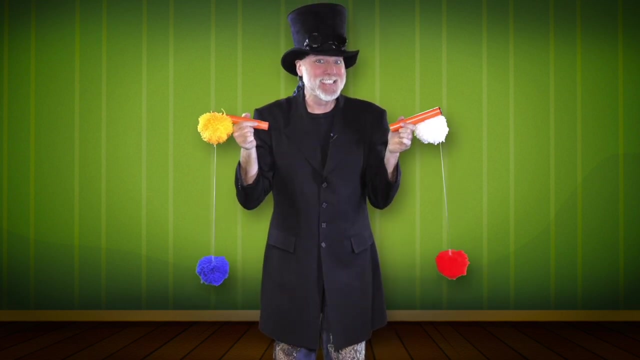 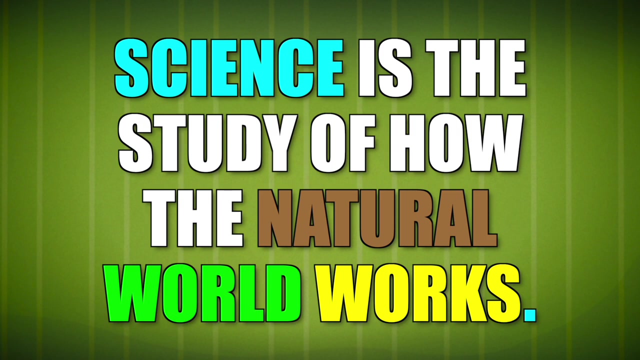 Magic is creating the illusion that you can defy the laws of nature. This is magic. Wow, Wow, Wow. Magic is creating the illusion that you can defy the laws of nature. Science is the study of how the natural world works. This is science. 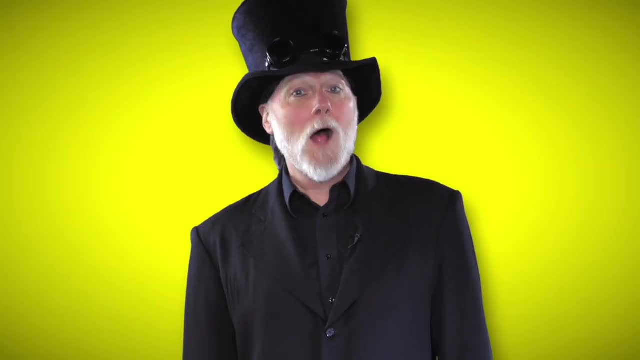 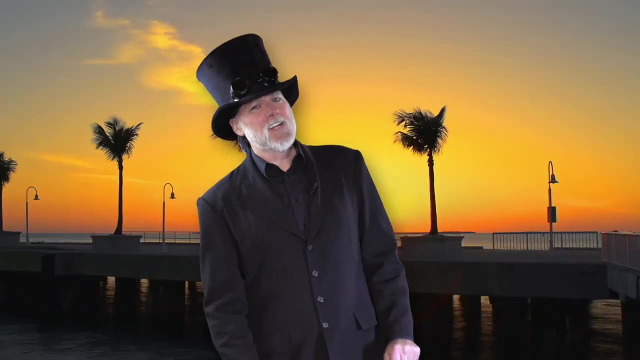 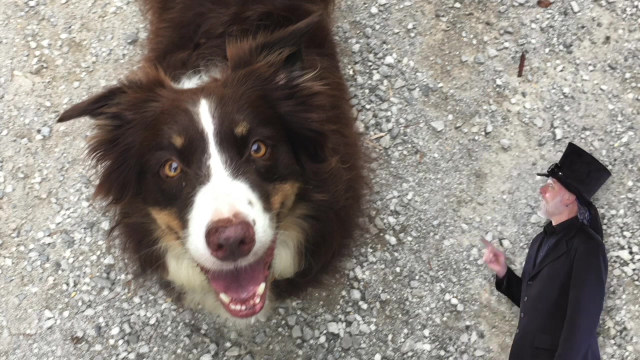 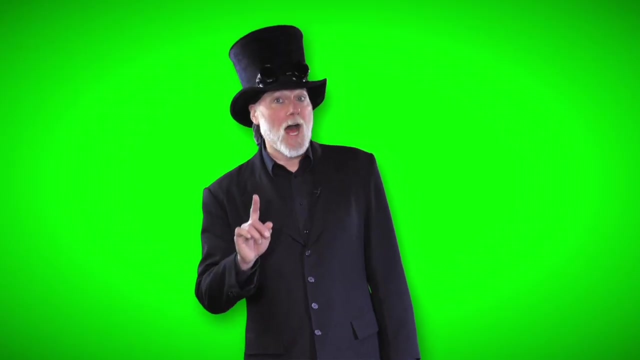 Wild, wild wildlife, Wildlife conservation. Wildlife is all around us. Wildlife traditionally refers to undomesticated animals, Not your pet hamster, Larry, Or my pet Australian shepherd Gracie. Wildlife includes undomesticated animals and all of the plants, fungi and other organisms that grow or live wild. 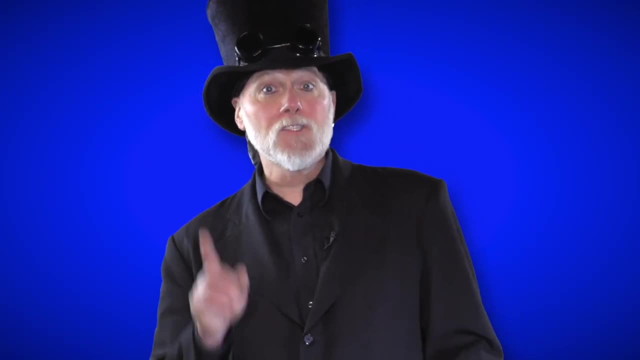 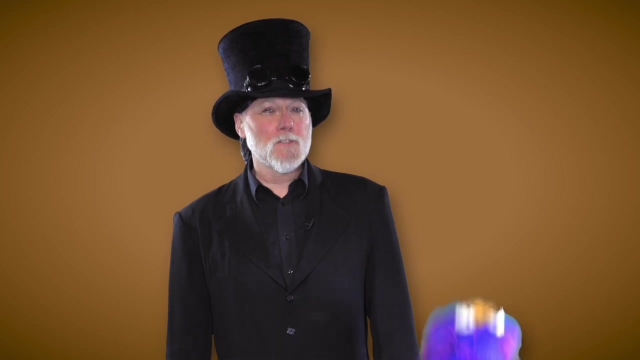 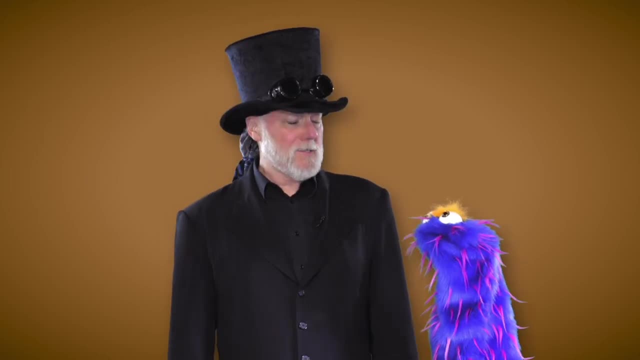 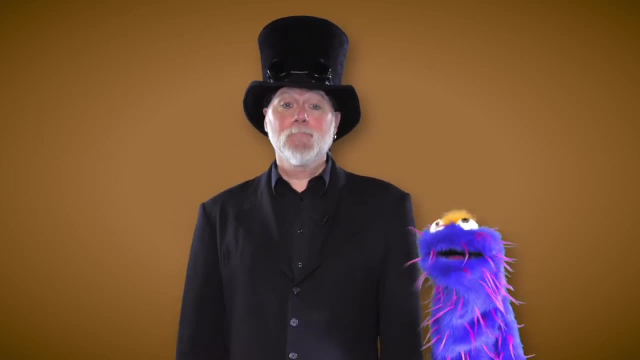 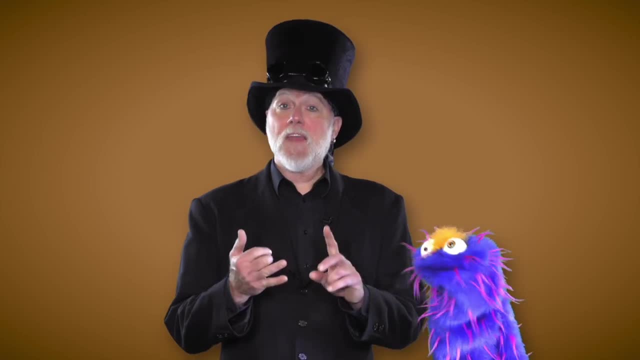 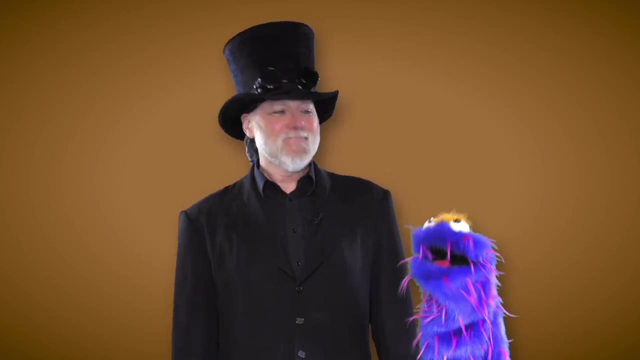 Well, because everything in the natural world is connected, The plants and the animals and humans all interconnected in this big huge web of life. plants and the animals and humans all interconnected in this big huge web of life. hmm, does that mean puppets too? well, that's an interesting idea. well, yeah, I. 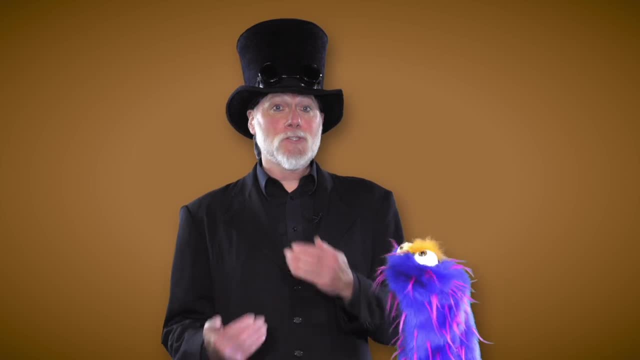 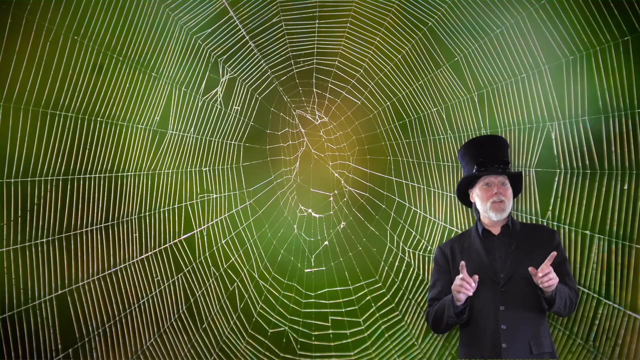 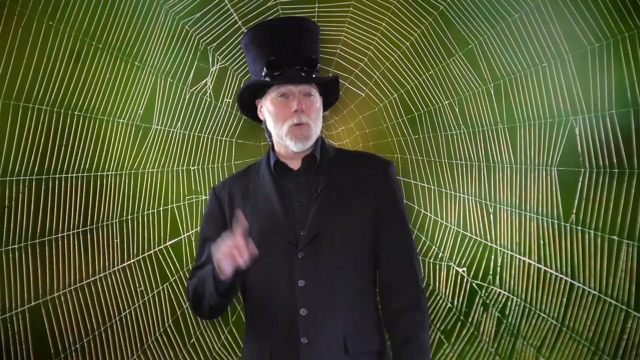 guess it does include puppets, because everything in nature is connected. so yes, that includes puppets too lovely. the web of life is like a giant spider's web because everything is connected to everything else. this means that the harm we do in one part of the web, even if we don't see that harm, can do harm in. 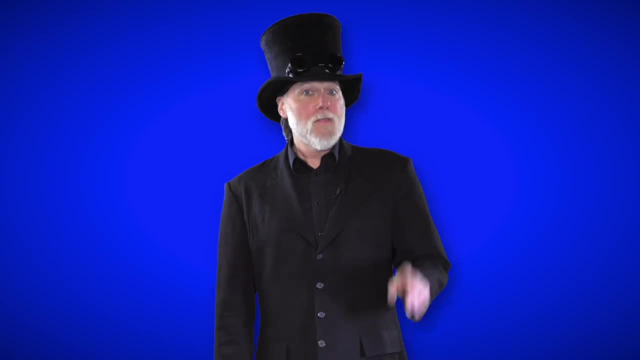 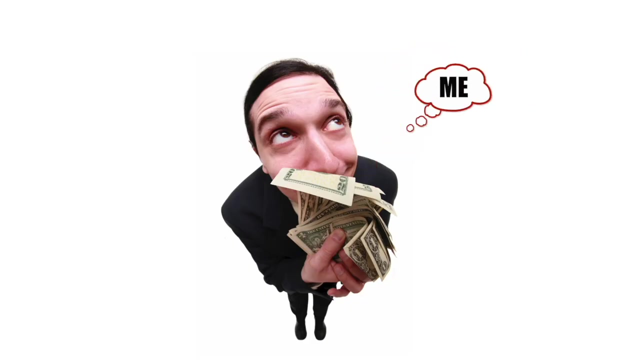 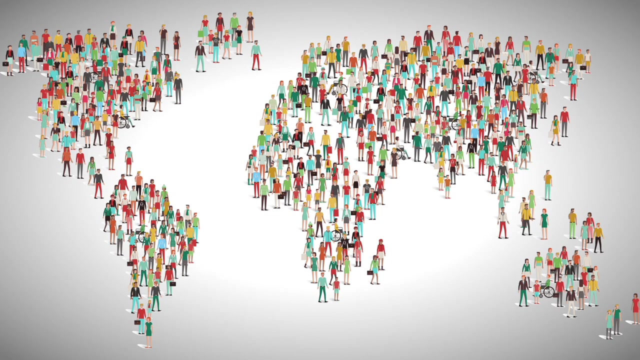 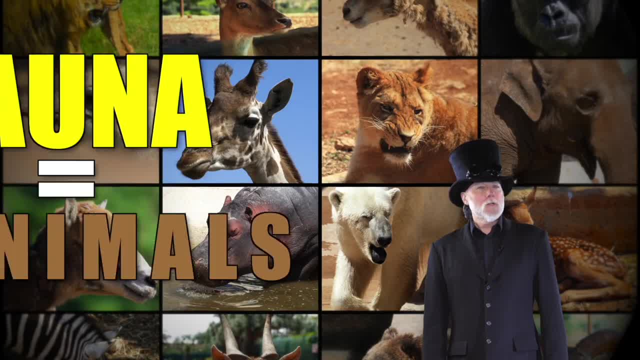 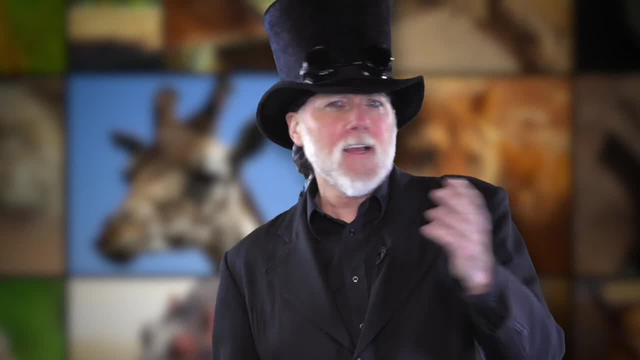 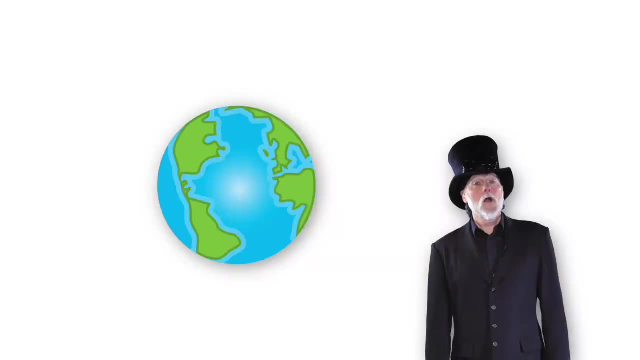 that are native to a particular region. not only does protecting wildlife add to our lives biologically, it adds a richness to our understanding of the natural world. humans sometimes forget that we are intimately connected to the earth and its systems. earth can live. without people, people cannot live. 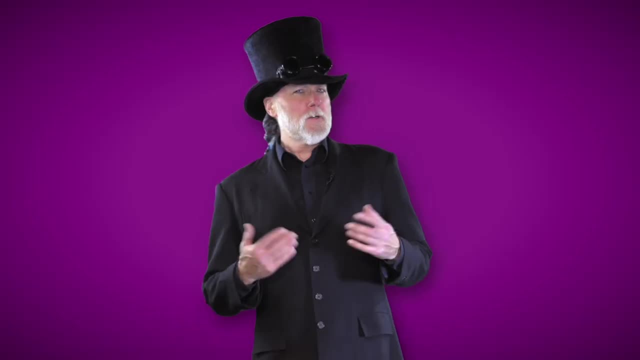 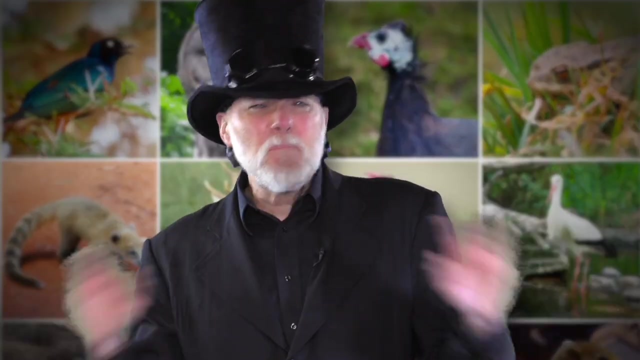 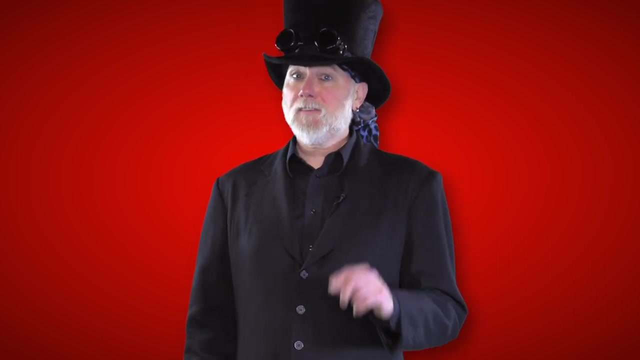 without earth. there's a kind of humility that people demonstrate when they help protect the vast, enormously, hugely bigly big variety of life on Earth. we are important, but we share the planet with lots of other important creatures as well. okay, so why are other living things important? first, all living. 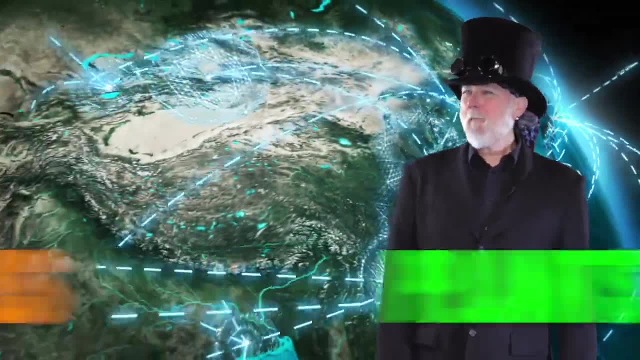 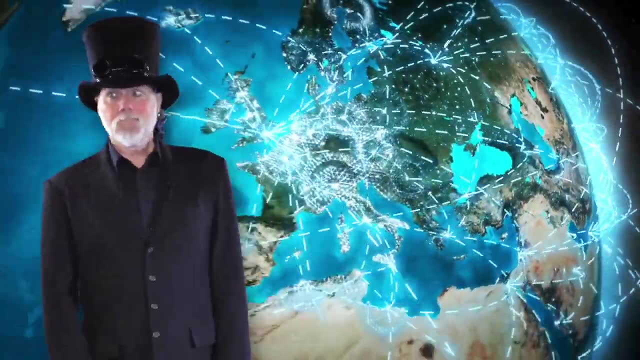 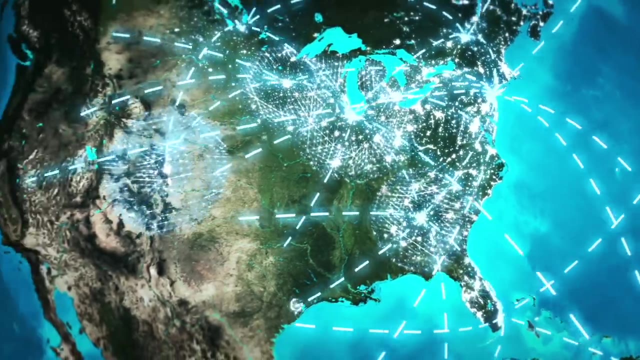 things on planet earth are a part of a system where everything is connected, and it has been that way for a very, very long time, well, really, since forever. it's how the system works: the air is connected to the water, which is connected to the soil, which is connected to the plants, which are connected to the animals. you 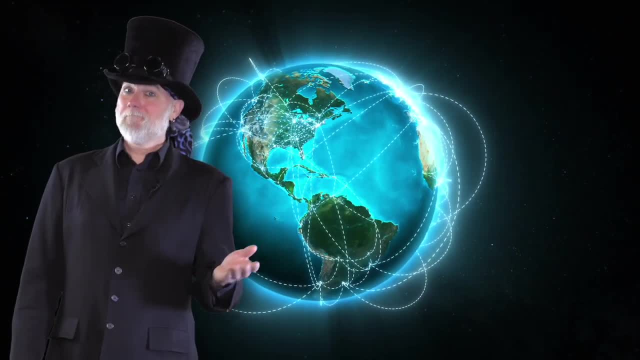 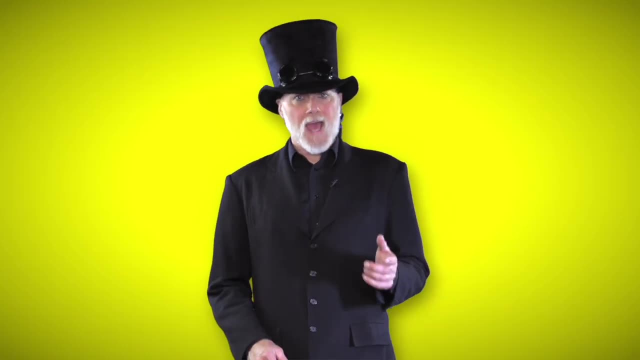 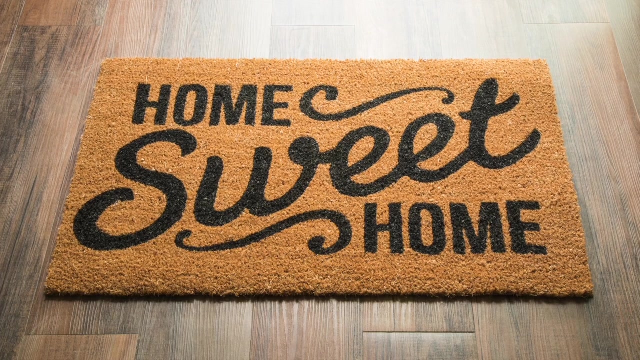 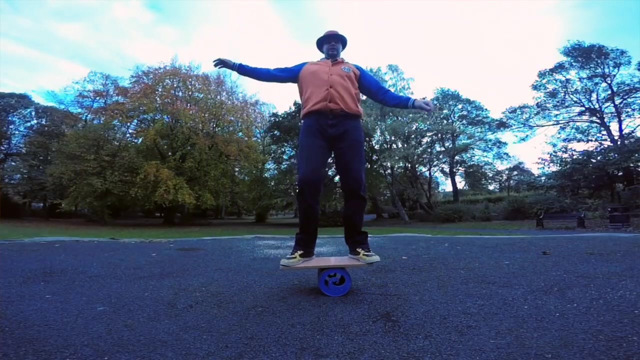 and I are animals, which is connected to the water, and on and on and on got it. everything is connected. the natural home of an animal, plant or organism is called its habitat. plant and animal organisms have adapted over huge spans of time to live in their specific habitats. interestingly, nature is always seeking. 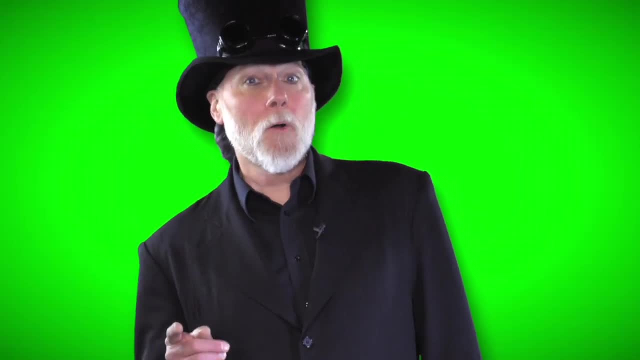 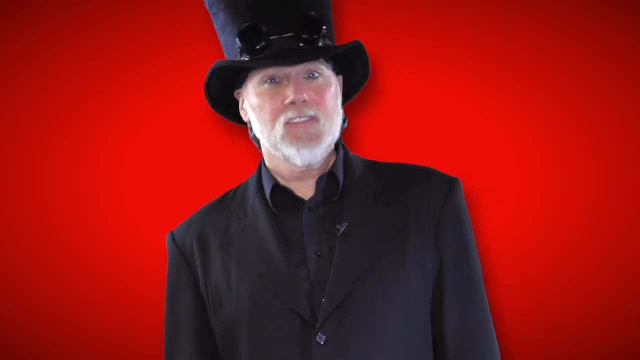 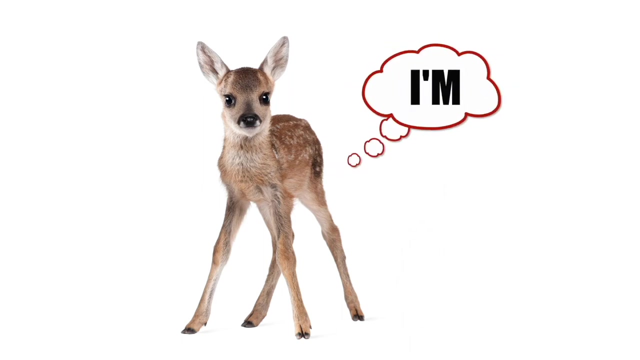 balance, even within established habitats. if one part of the system gets out of balance or out of whack, it will affect the other parts. sometimes we can't even predict what the effect will be. here's a simple example: dear, beautiful, fast, adorable. a balanced number of deer in one area controls the vegetation, or plants in that area, but too many deer might eat all of the plants in their habitat. the system becomes unbalanced. when the deer move out of their habitat looking for food, their new food source might be the plants in your yard or a farmers field of corn. this can be a 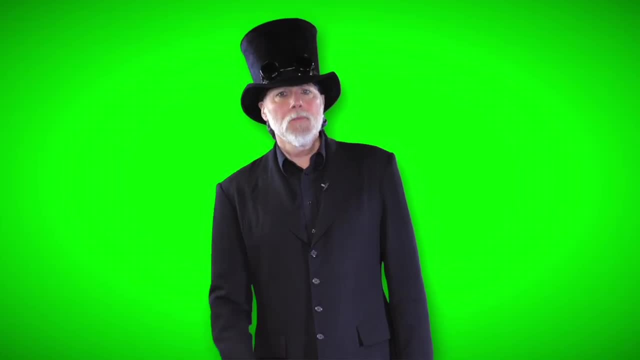 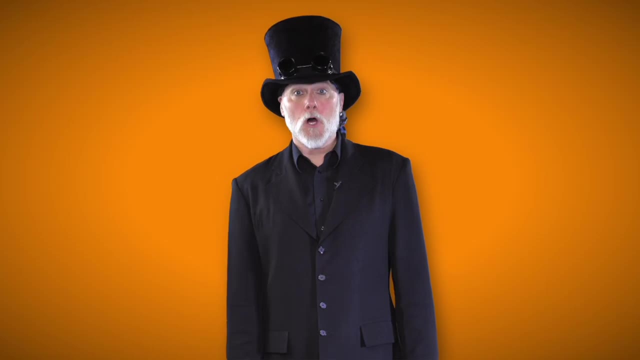 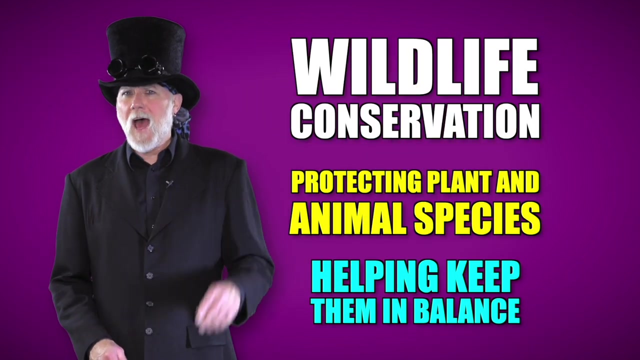 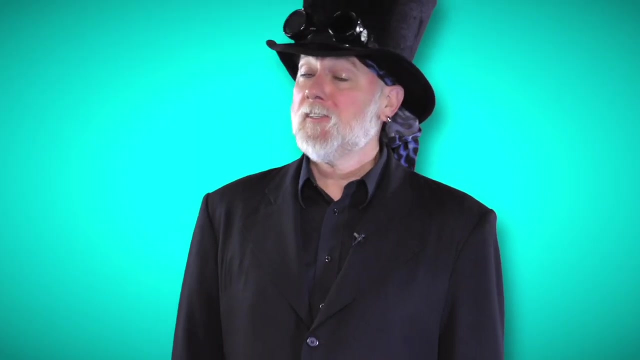 problem causing an imbalance. however, the opposite of this can also be true. too few deer can allow the vegetation to grow over, and that can also cause imbalance. wildlife conservation is protecting plant and animal species in their habitat and helping keep them in balance. equilibrium is another word for balance. this balance isn't just for deer. it. 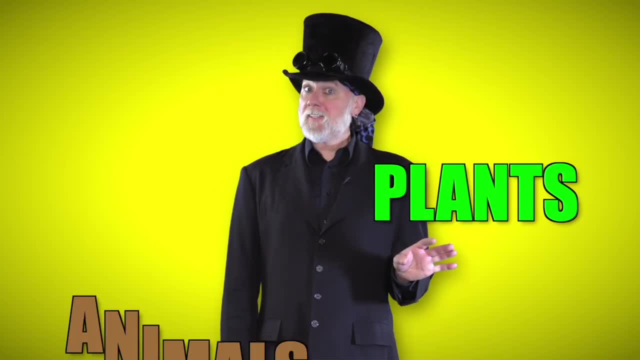 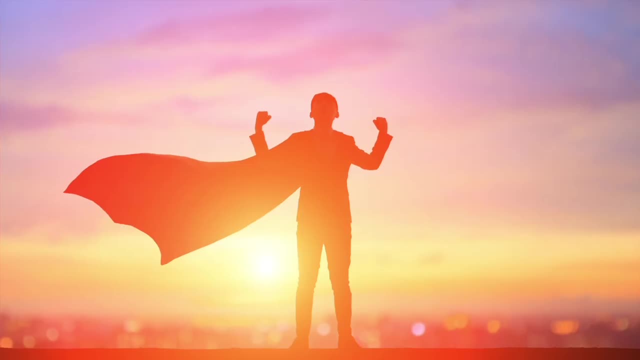 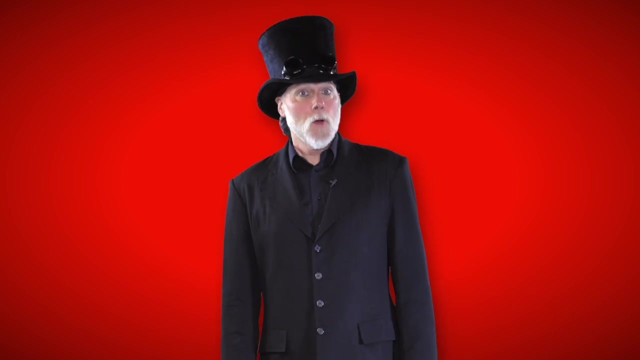 applies to all wildlife. native species include all of the plants and all of the animals that call a region home before humans began interacting with that habitat. humans are very powerful and can change habitats, harm wildlife and harm native species, even if we don't mean to, and because this is so, it also means that 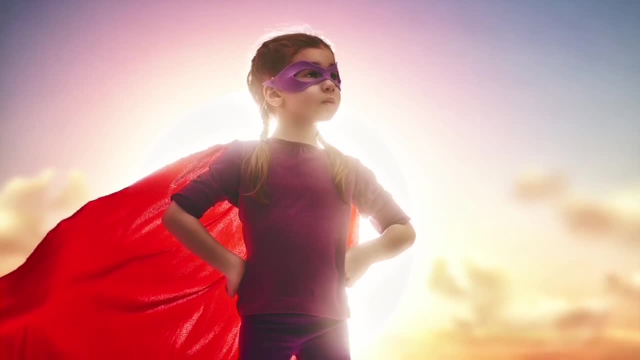 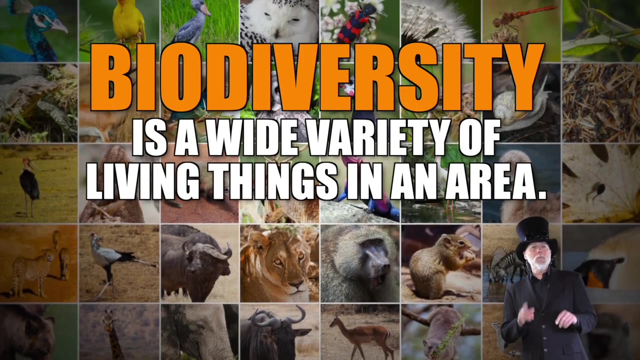 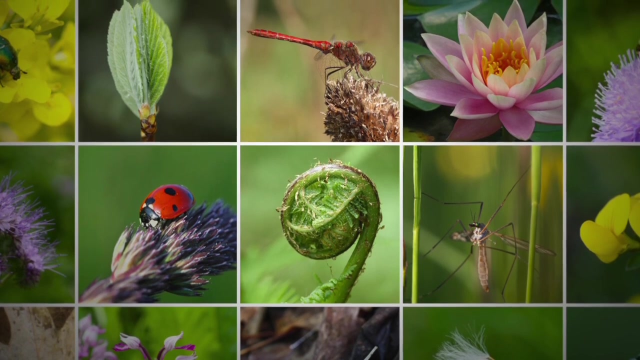 humans are powerful enough to conserve and preserve their habitat, and also to protect wildlife biodiversity. biodiversity is a term that describes the wide variety of living things in an area. if one plant family is wiped out by disease, a similar plant family in the same area may survive and balance can. 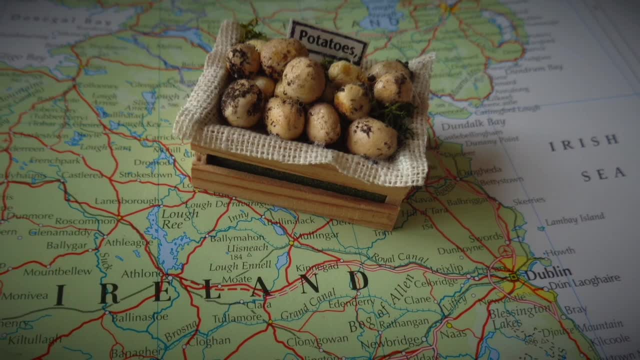 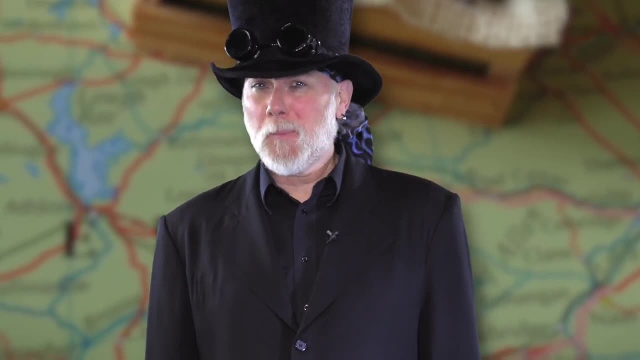 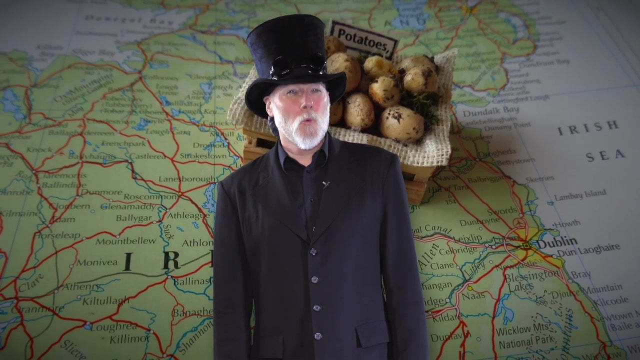 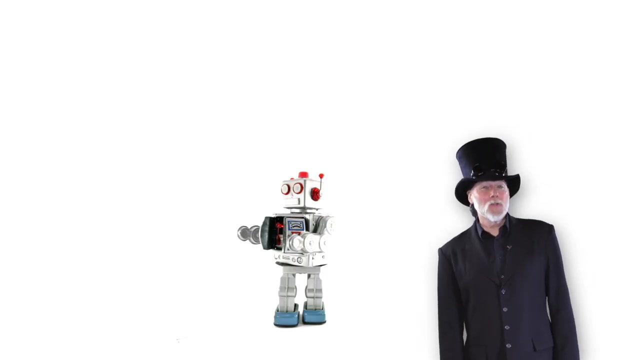 continue. the great potato famine of 1845 in Ireland caused many people to starve to death because they only had one variety of potato plant for food, when that plant couldn't resist a widespread disease. many, many, many people suffered. wildlife can be an extremely important environmental indicator. it can show us a problem that needs to be fixed for 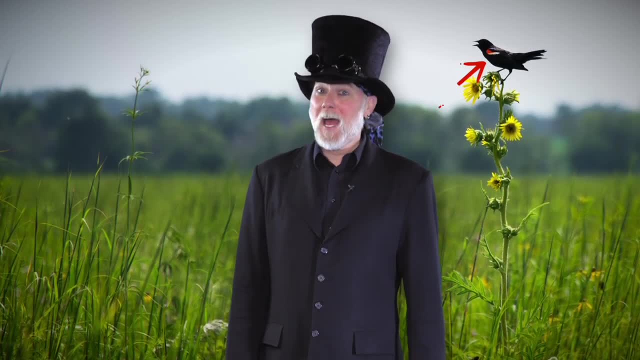 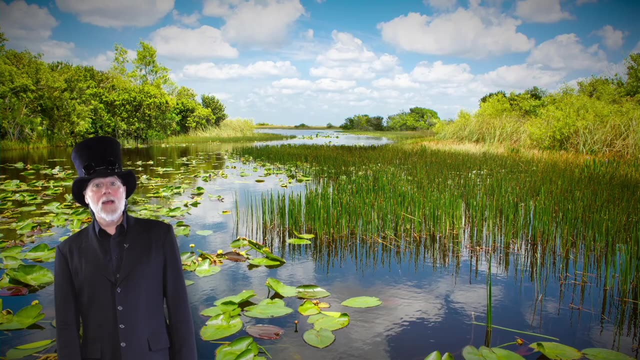 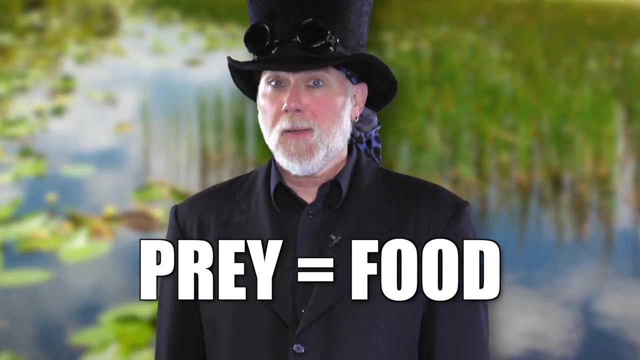 instance, wild birds are dependent on a healthy habitat. the population of birds going up or down can tell us a lot about how well the system is functioning. for example, numbers of wading birds nesting in the Everglades are dependent on prey. their food availability- the prey can depend on. 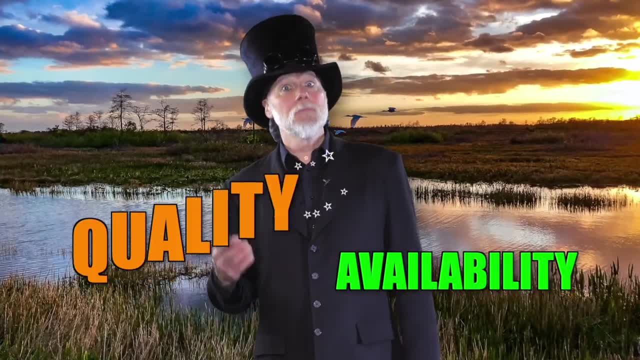 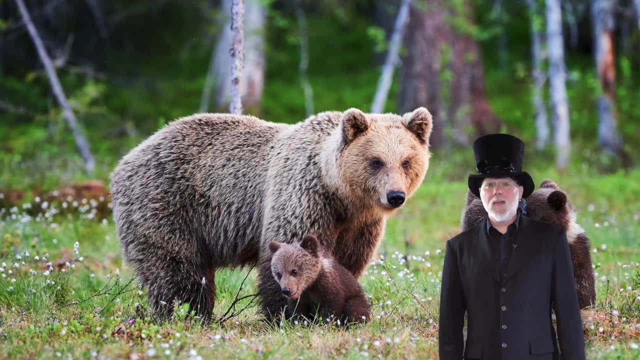 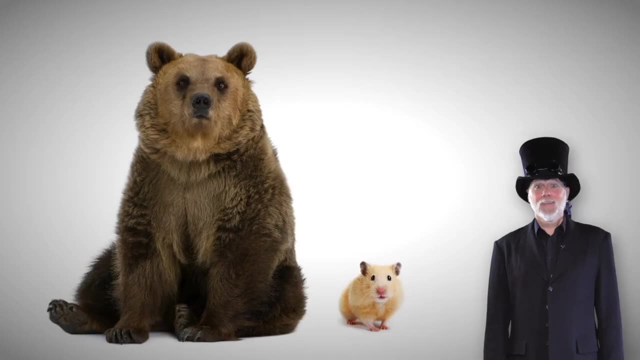 many factors, including water availability and water quality. wildlife contains unique and valuable things that cannot be replaced when they're gone. protecting wildlife may even have undiscovered health benefits for humans. some scientists believe that bear saliva- yeah, bear saliva- has a powerful antibiotic. oh, there is so much undiscovered knowledge in the